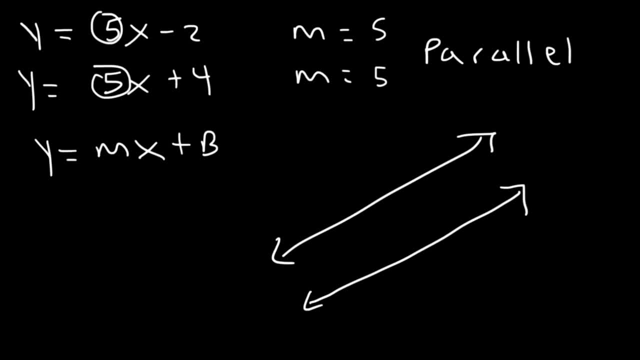 other. They have the same slope and, as a result, parallel lines will never intersect. Now, what about these two equations? How would you describe the relationship of the graphs of these two equations? So the slope for the first one is positive, 2 over 3.. For the second one, 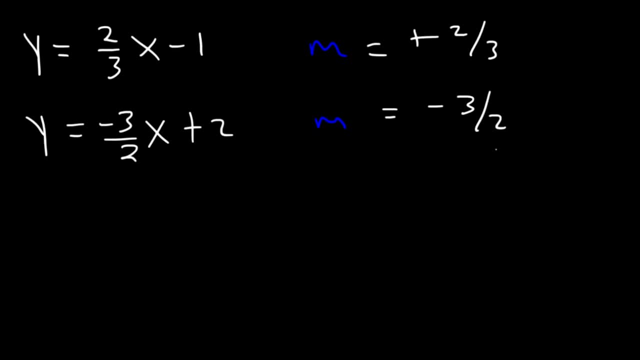 it's negative, 3 over 2.. Whenever the two slopes, if they're inverses of each other, they're inverses of each other. Well, I'll take that back. If they're the negative reciprocals of each other, then 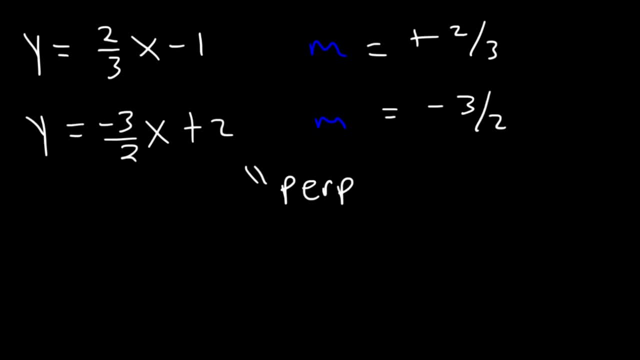 they're perpendicular. So, for instance, let's say if the slope of line 1 is positive- 4 over 3.- The perpendicular line will have a slope of negative, 3 over 4.. You need to do two things: Flip the fraction, change the sign. 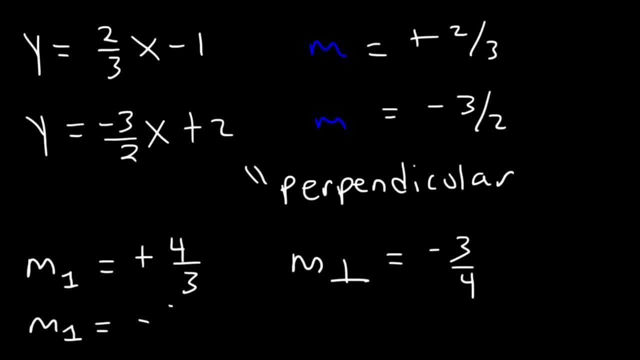 Now let's say if the slope of the first line is negative, 7 over 5.. The slope of the perpendicular line is positive, 5 over 7.. Now you need to know that a perpendicular line intersects another line. at right angles This is going to form a 90-degree angle. If you were to graph it, that's how. 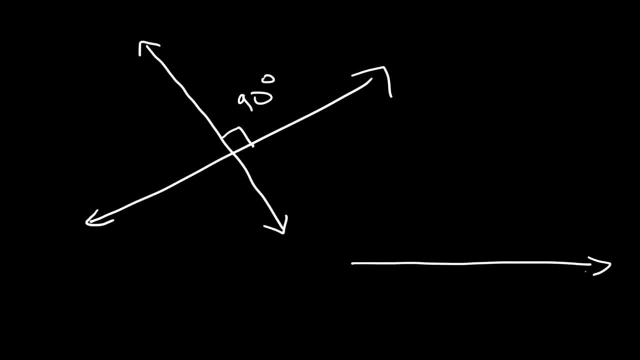 it's going to look like. So let's say, if you have a horizontal line, A line perpendicular to a horizontal line is a vertical line and it's going to form a 90-degree right angle. So those are some properties of perpendicular lines. Now what about this one? Let's say 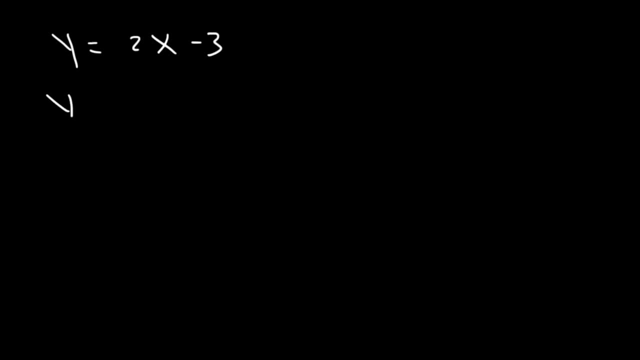 if Y is equal to 2x minus 3, and also 3x plus 1, what's the relationship between these two lines? Are they parallel, Perpendicular Or neither? So first notice that the slope is not the same, so it's not going to be parallel to each other. now, if we take 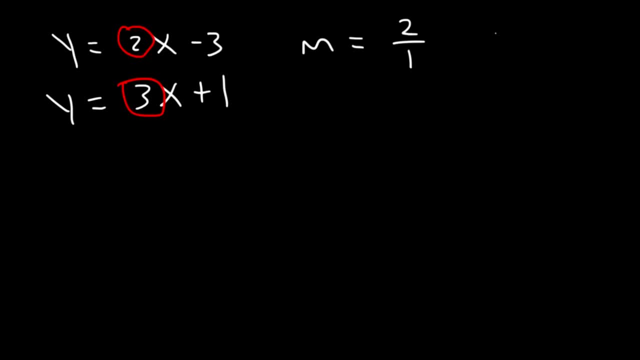 the first slope which is 2 or 2 over 1, and if we find a slope that's perpendicular to it, which is going to be negative, 1 over 2, don't forget to change the sign and flip the fraction. notice that this slope is not the same as 3. 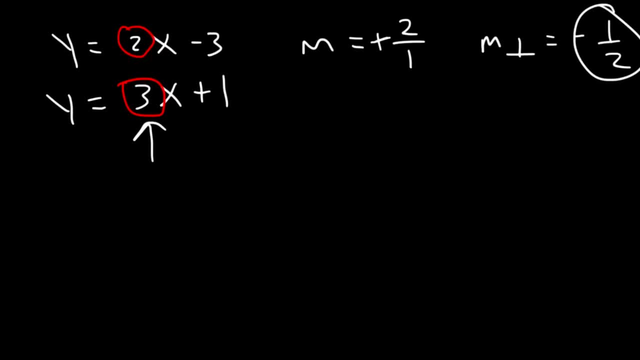 therefore, these lines are not perpendicular, which means that it's neither they're not parallel and are not perpendicular. so just to review, parallel lines have the same slope. perpendicular lines have slopes that are negative reciprocals of each other. so the first slope is, let's say, 6 over 7. the other one is going to: 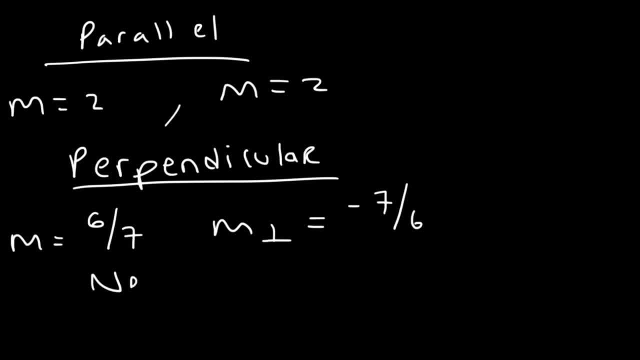 be negative: 7 over 21 over 6.. And if it's not one of these two, then it's neither. 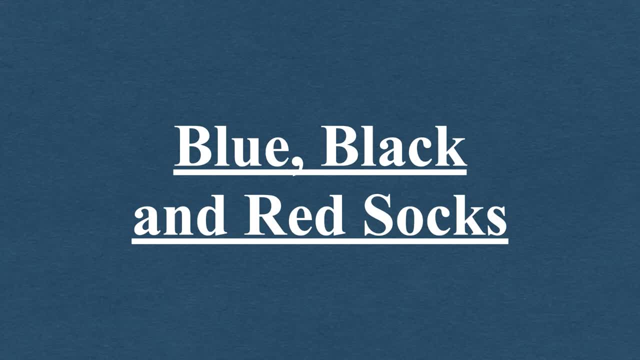 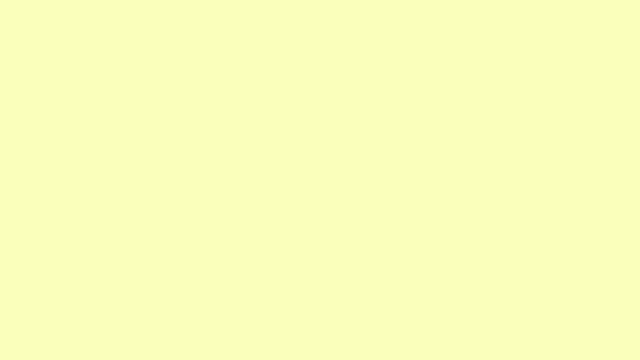 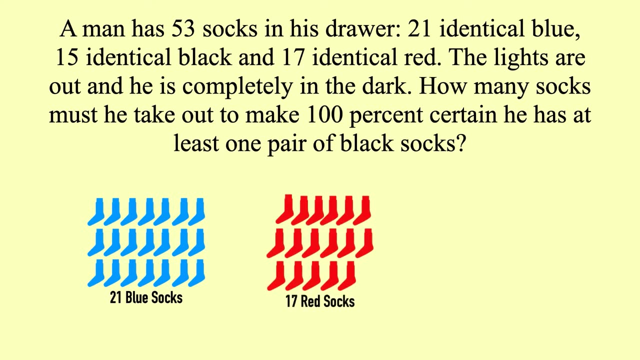 Welcome to Simply Logical. this is Venkatesh. In this video, let's check one of the most interesting riddles. A man has 53 socks in his drawer: 21 identical blue, 15 identical black and 17 identical red. The lights are out and he is completely in the dark. How many socks must he take out? 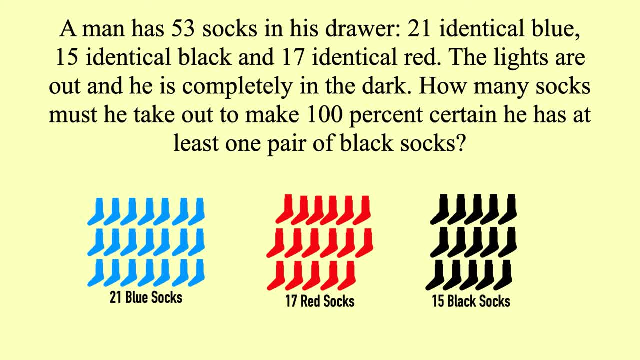 to make 100% certain he has at least one pair of black socks. This is one of the most interesting recent riddles to surface online. But what exactly is the answer to this puzzling problem? Feel free to pause the video and try yourself before. 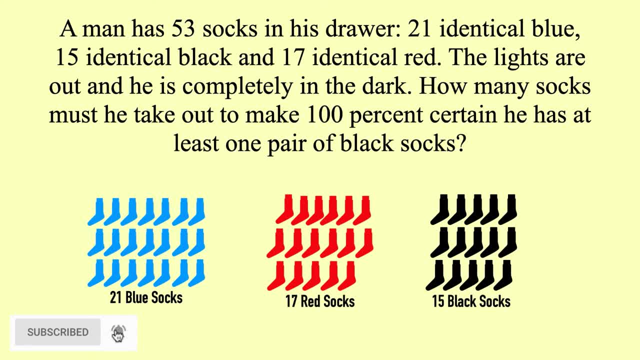 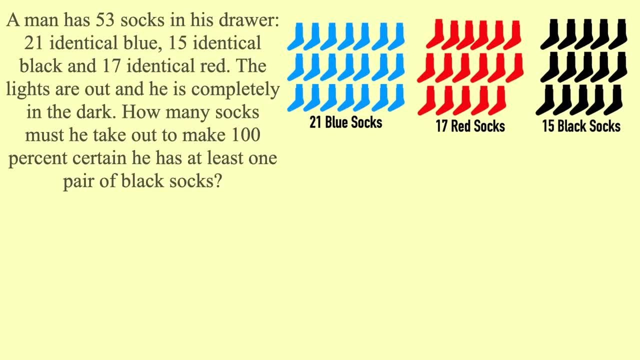 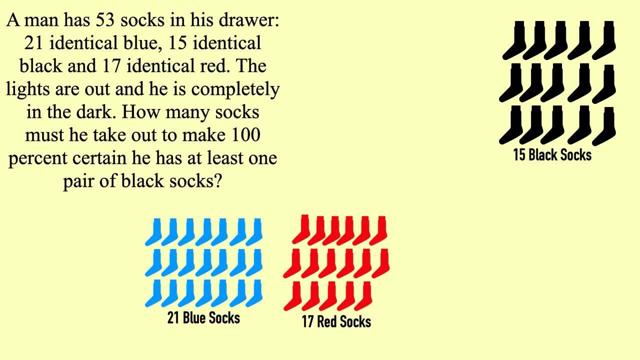 checking the solution. Let's everyone know your answer in the comment section. So let's check the solution now. The answer to this puzzle is 40 socks. If he takes out 38 socks adding the two biggest amounts, that is 21 and 17,. although it is. 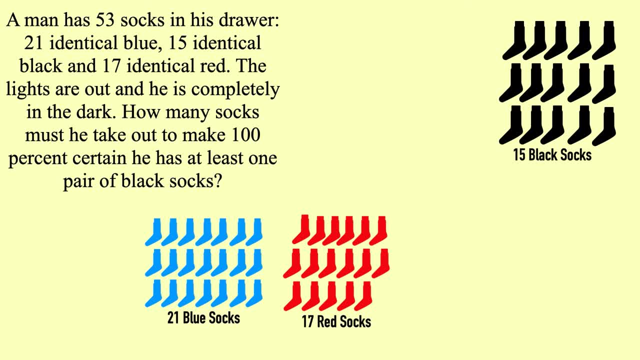 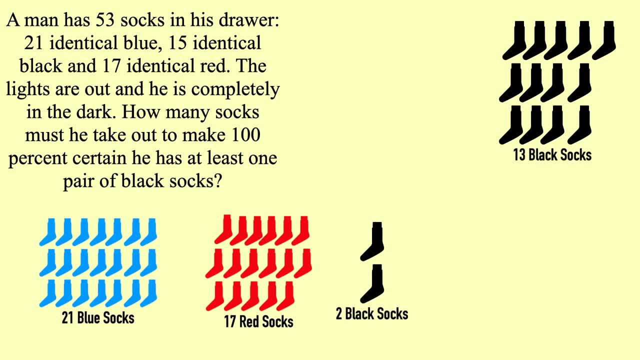 very unlikely. it is possible they could all be blue and red. To make 100% certain that he also has a pair of black socks, he must take out a further two socks, which results in 40 socks. By doing so, he will make sure that he will get at least one pair of black. 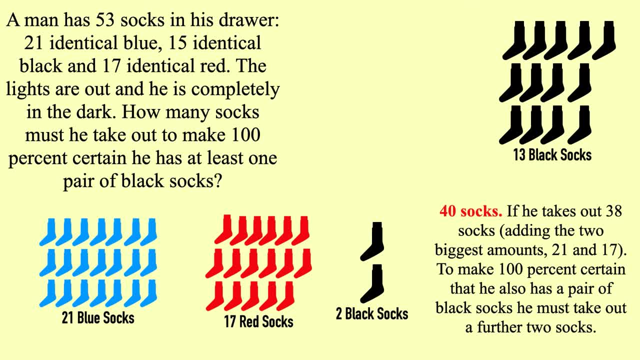 socks. That's all for this video. If you are new to the channel, please subscribe to the channel. Let's meet in the next video. Thanks for watching and thank you for your support.